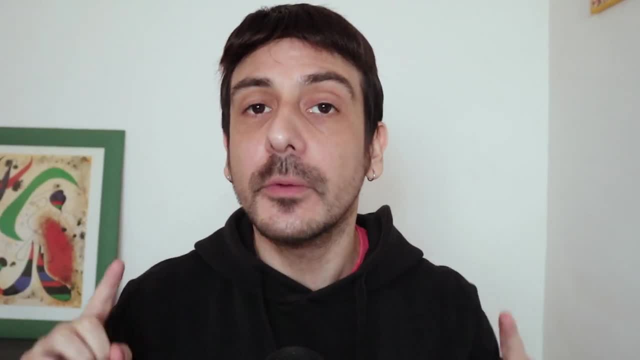 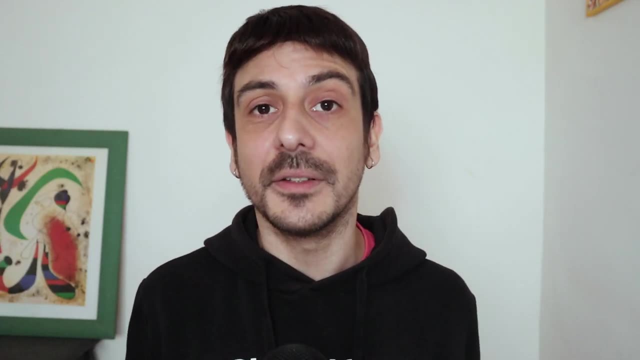 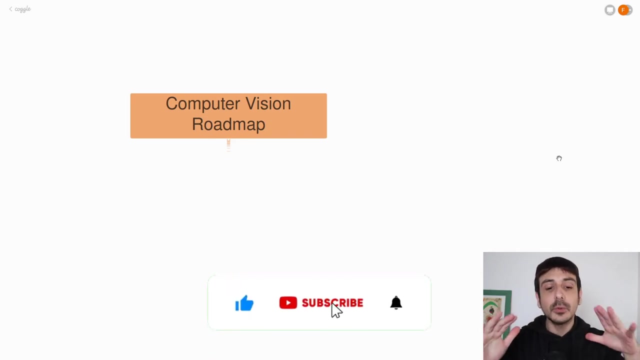 computer vision, And I'm also giving you very specific resources you can use in order to learn all the skills I show you in this roadmap. And now let's get started. So let's get started with this computer vision roadmap. In this video, I'm going to show you an entire roadmap in order to 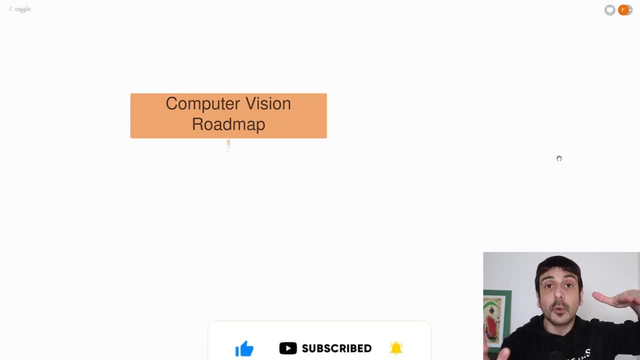 go from zero from scratch, from having absolutely no background in IT whatsoever up to a complete expert computer vision engineer. So let's get started. The first step you should follow in this roadmap is covering the fundamentals, And when I say fundamentals, I mean Python and OpenCV. 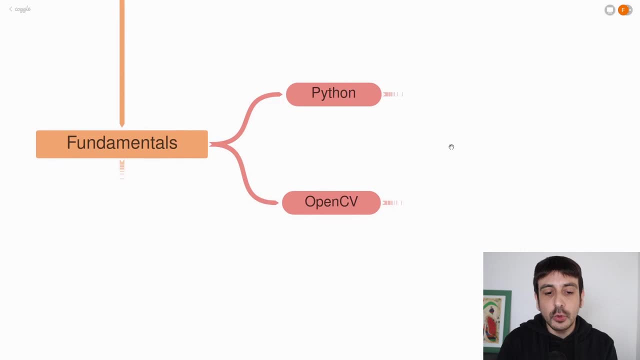 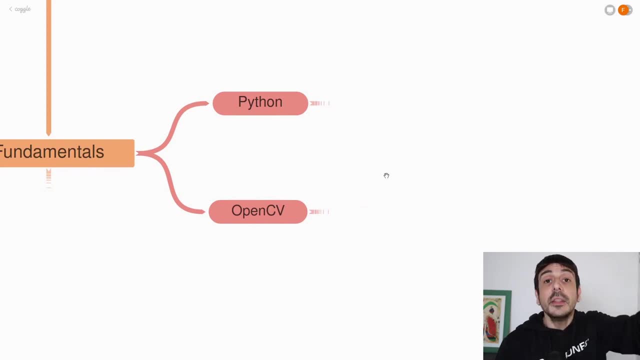 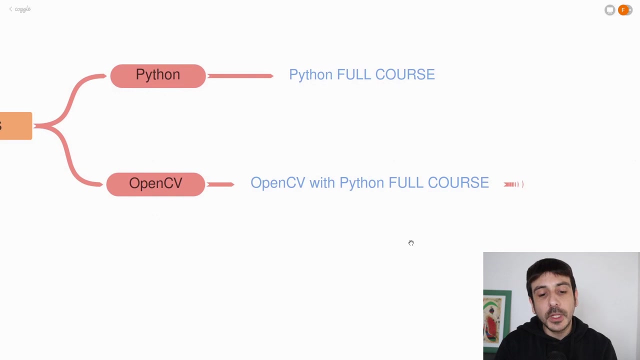 And this video, this computer vision roadmap, is an updated version of one of my previous videos And in this version I have added some specific resources you can take, you can follow, in order to learn all the different skills I am going to show you in this roadmap. So, in order to learn, 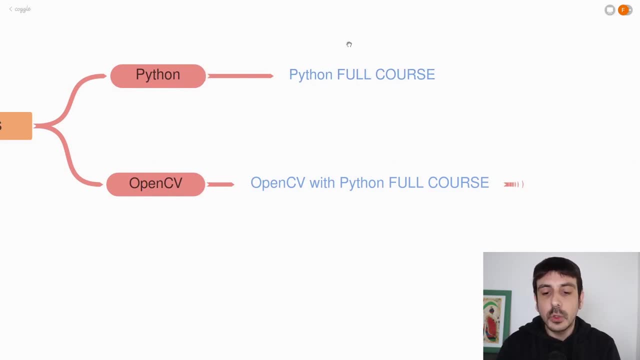 Python and in order to learn OpenCV. you can take a look at these two resources I have added over here. And regarding OpenCV, this is a three hours long fully comprehensive course of OpenCV with Python And I definitely recommend you to check out this course, But if you do not, 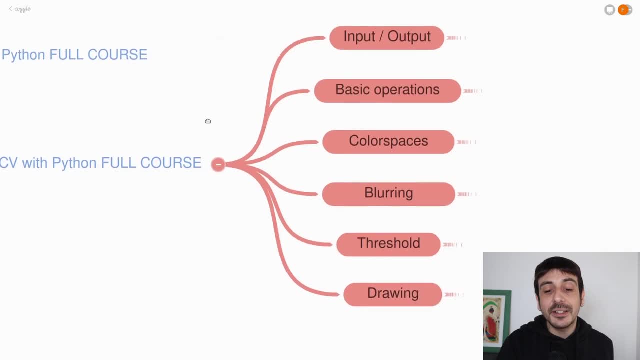 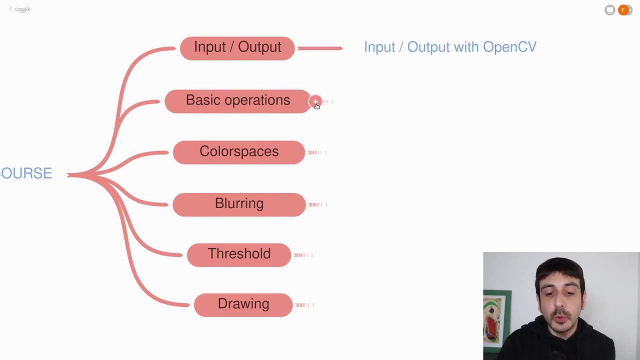 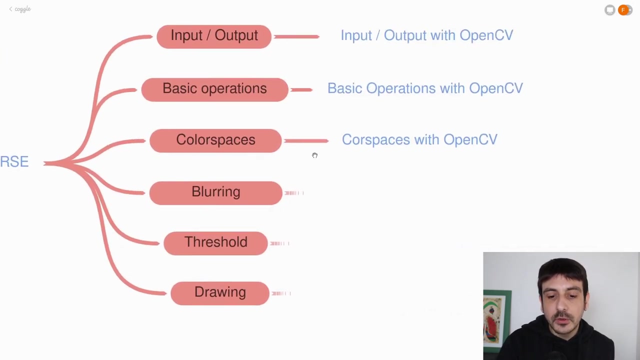 have three hours in order to take this course, then these are the most important lessons you should take in order to cover the basics of OpenCV with Python. So if you do have three hours, then please take a take a look at this course. But if you do not, don't worry, you can just take. 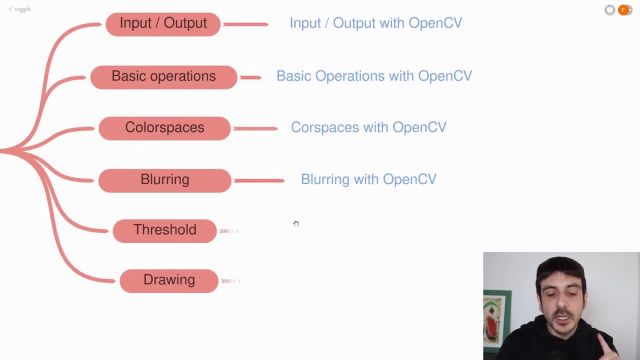 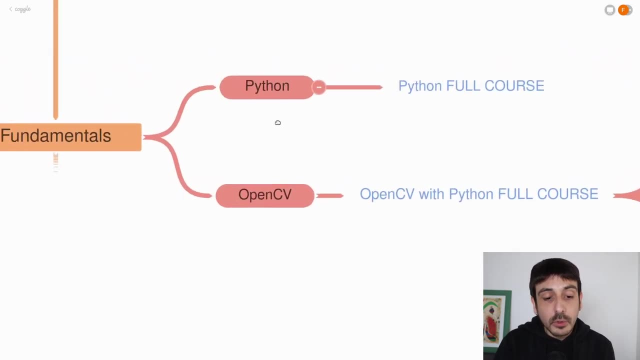 some of these lessons and you are going to cover the most important aspects of OpenCV with Python. So this is the first step you should take in order to learn computer vision, in order to become a computer vision engineer. And now let's continue. The next step in this roadmap is the basics of 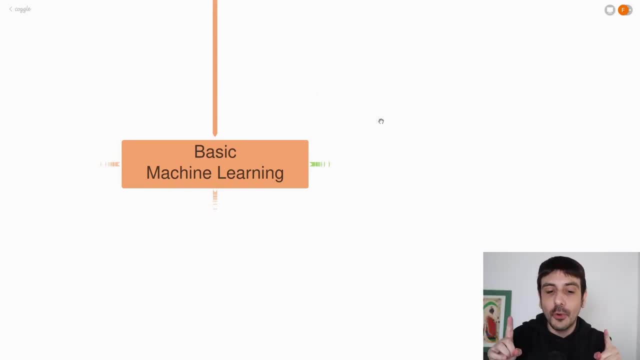 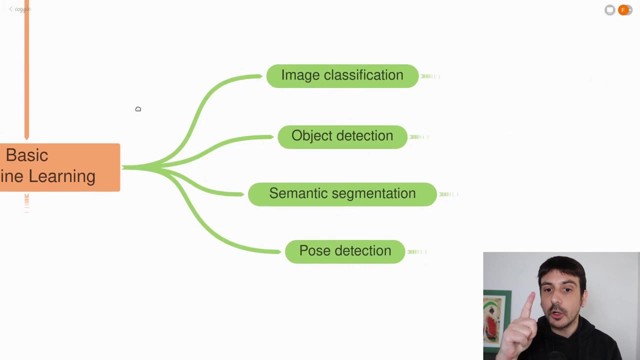 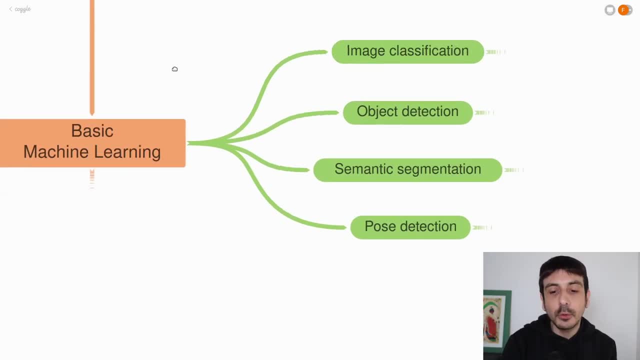 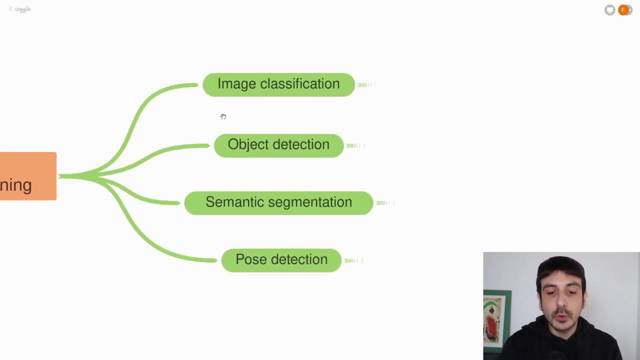 I recommend you to learn machine learning by learning how to solve these four very specific problems, these four very specific tasks. So, by learning how to build an image classifier, how to build an object detector, how to build a semantic segmentation algorithm and how to build a post detector, Oh my God, you will have learned so much machine learning. 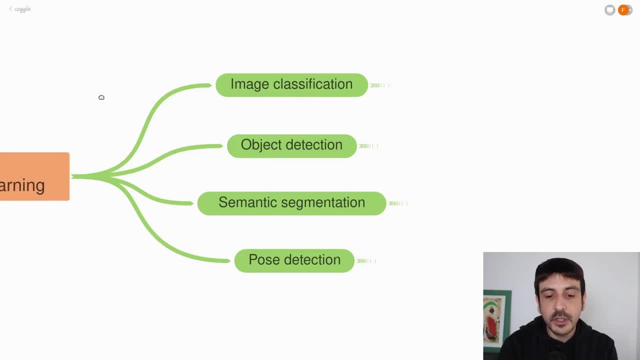 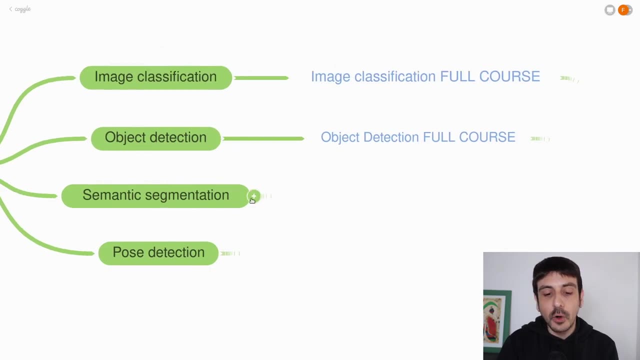 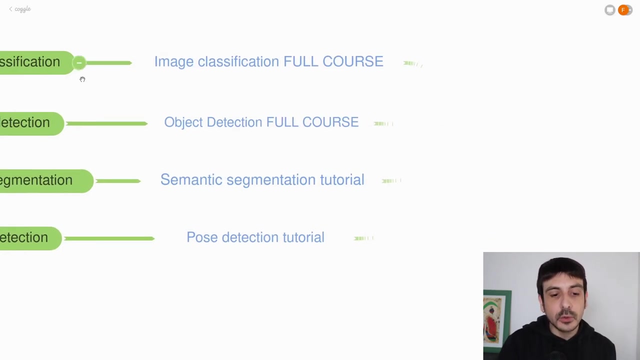 and you will be super, super proficient in machine learning. These are the most important specific resources you could use in order to learn how to solve these problems right. These are some courses and some tutorials I recommend you in order to solve these problems, in order to learn. 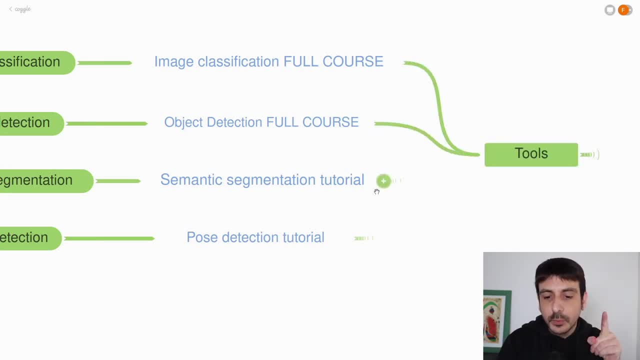 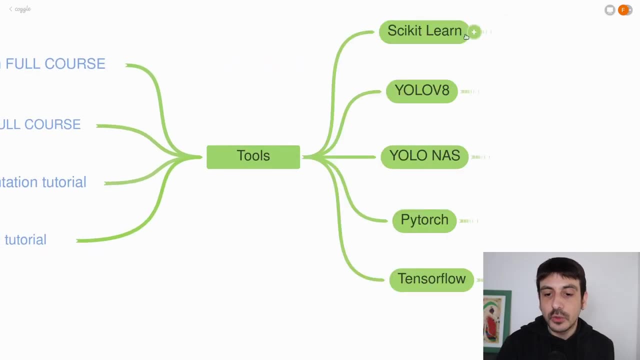 how to solve these problems And by doing so, by solving these problems, you are going to learn how to use some very specific tools, which are, let me show you, CKIT: Learn YOLO V8, YOLO NAS. 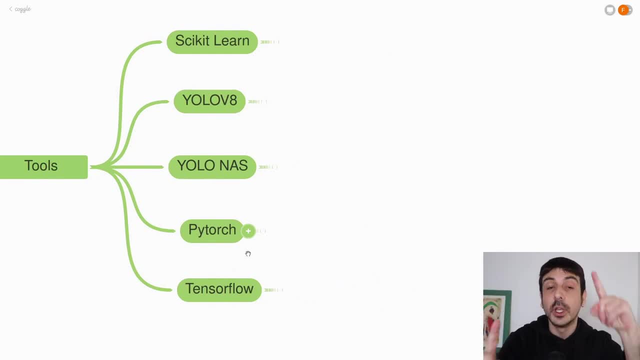 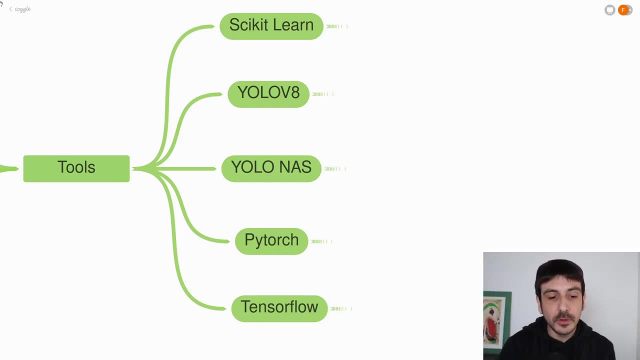 PyTorch, TensorFlow and many, many, many more tools, And please pay attention, because this is very, very, very important. These are the tools we use in order to solve these problems right, But the important thing is not the tools we use. The important thing 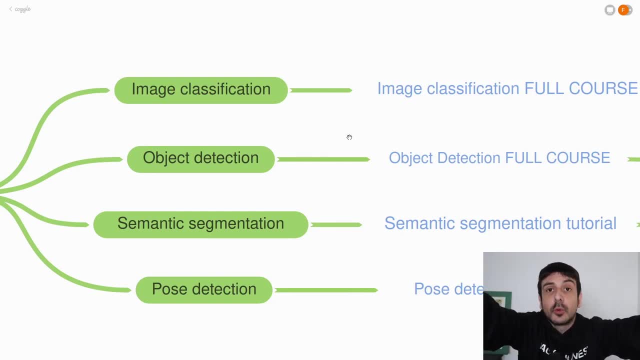 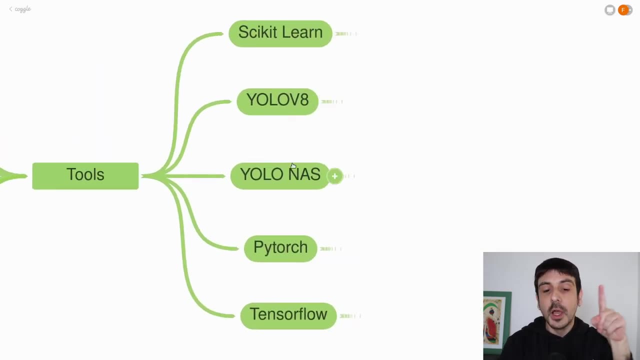 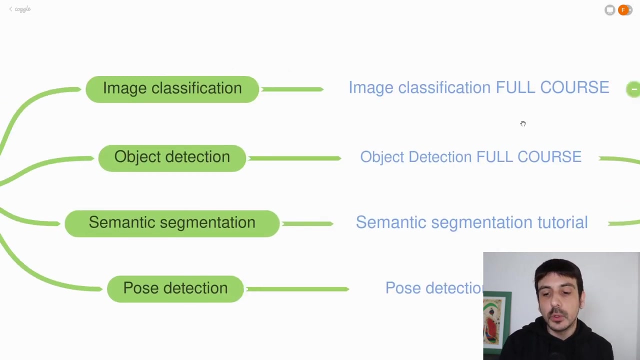 is the problems we are solving by using the tools, right. So my recommendation for you is: do not focus on learning how to use the very specific tools, but focus on how you are going to solve each one of these problems, And by doing so, you are going to learn how to use different tools. 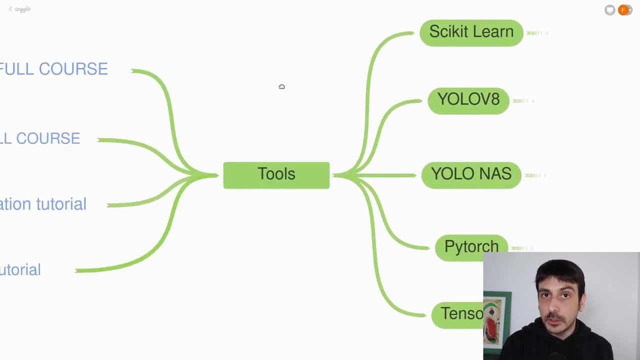 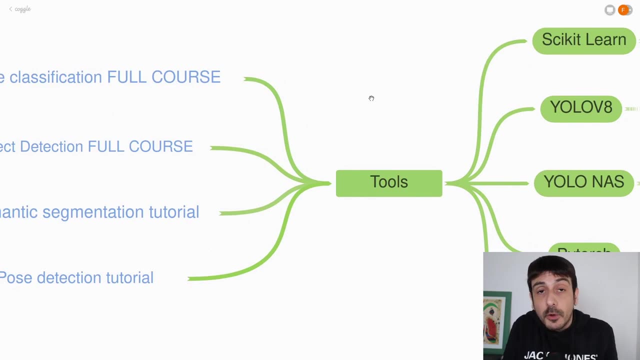 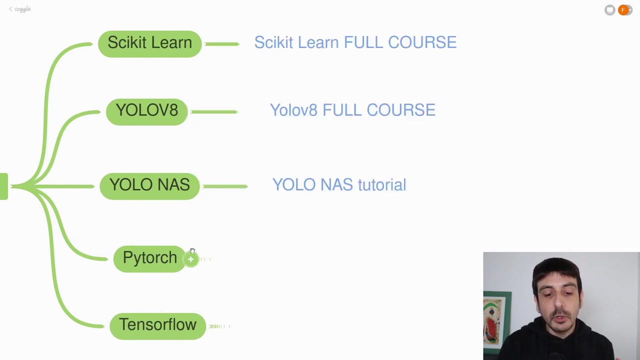 Right, My recommendation for you is: do not focus on learning the tools. focus on learning how to solve these very specific problems, But if you are one of those people who prefer to learn the tools, that's perfectly fine. I have also added some resources for you, right, Because I know we all 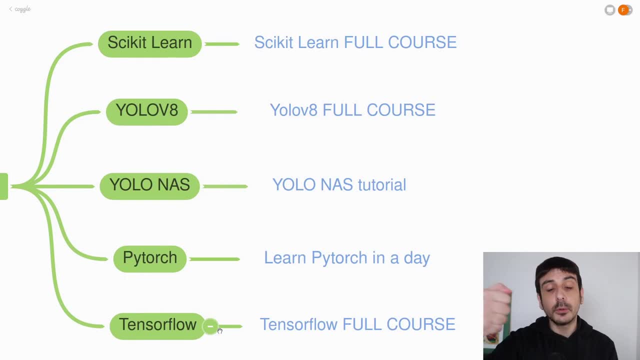 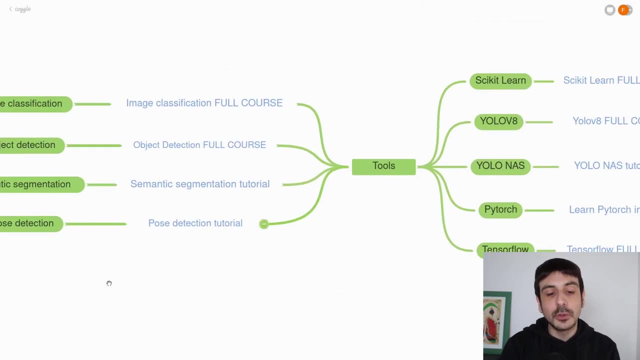 have different preferences. So if you prefer to learn how to use the tools, these are some resources you could use right. But remember, my recommendation is: do not focus on the tools. focus on how you're going to solve these problems And by doing so, you are going to learn how to. 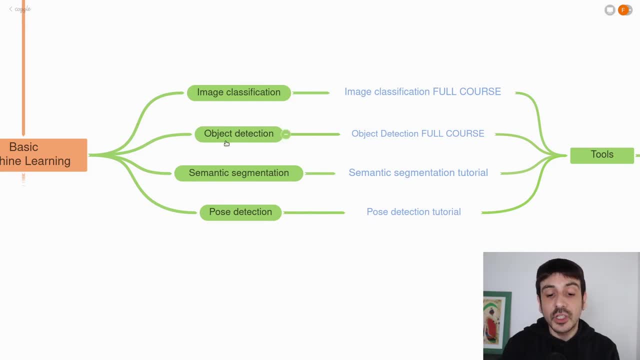 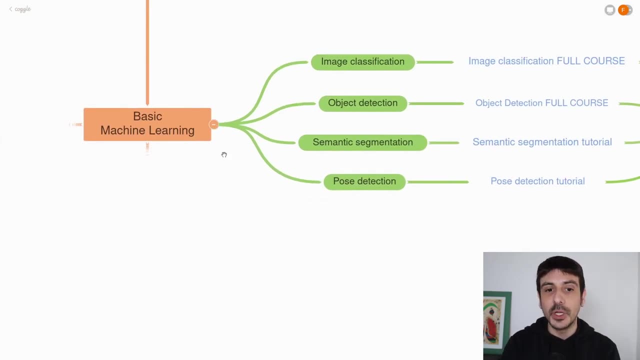 solve the high-level problems, image classification, object detection, semantic segmentation and pose detection, which are perhaps the most important machine learning problems in computer vision. Now let's continue, And you can see that from here, from basic machine learning, you can. 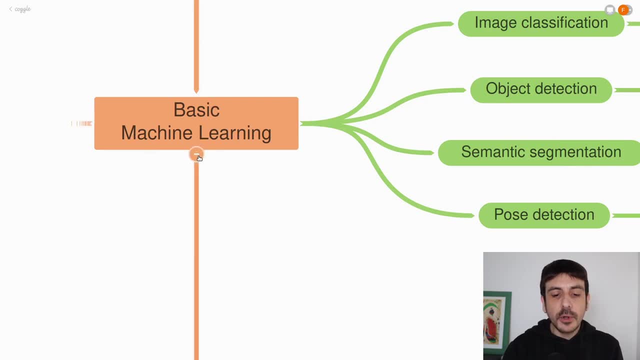 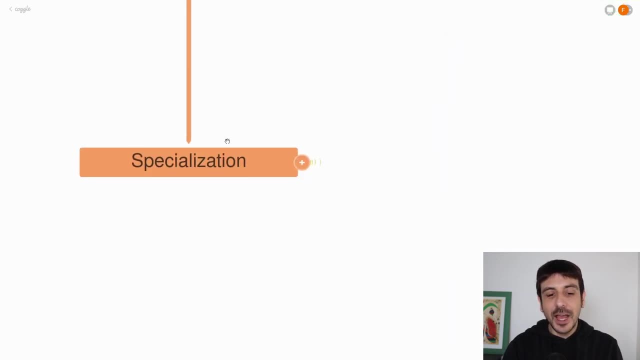 take it in either one of these two paths. Let's take it over here for now, And later on I'm going to show you what's over here. So, following this path, we have the specialization. right Now that you feel better, you can take it over here And then you can take it over here, And then you can. 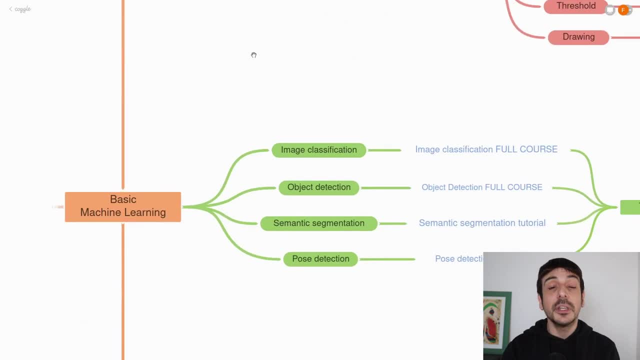 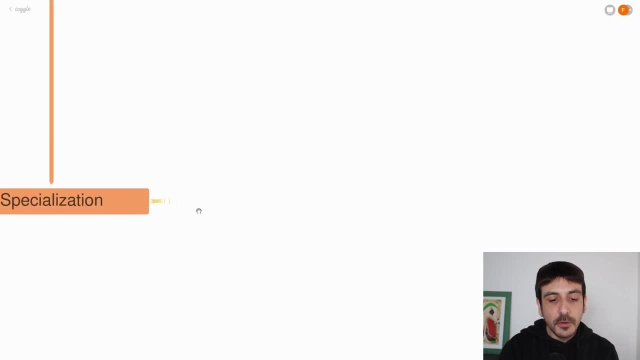 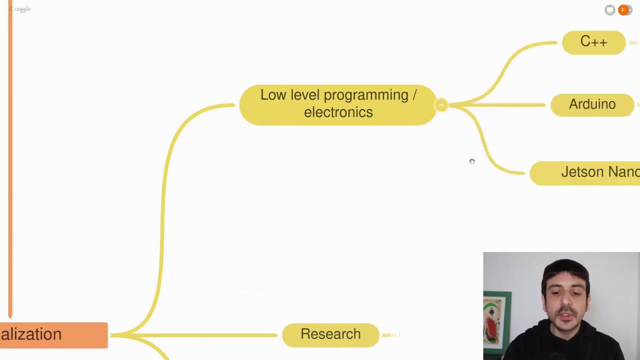 now it's time to specialize right, And you have many different ways to specialize. One of these different ways is low-level programming and electronics, which basically involves C++ and how to work with an edge device, for example Arduino or Jetson Nano, And the reason this is 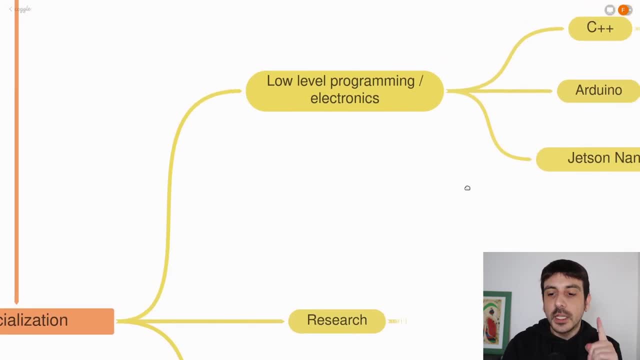 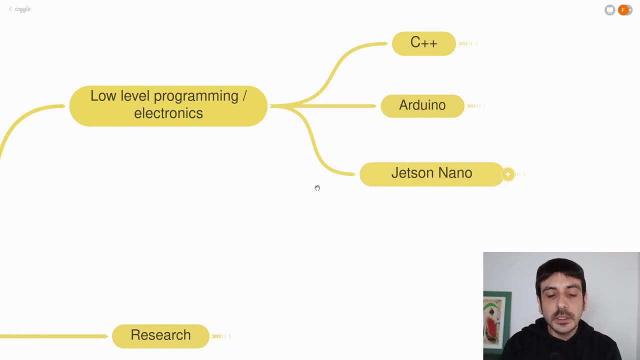 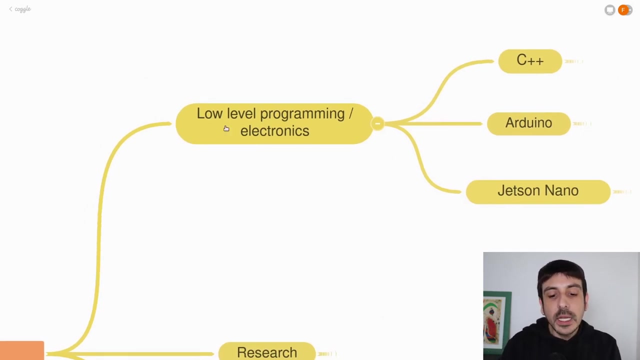 one of the ways in which you can specialize in computer vision is because, although C++ is a very, very, very important programming language, you can definitely take up many projects as a computer vision engineer, and you can just become a computer vision engineer without really doing anything. 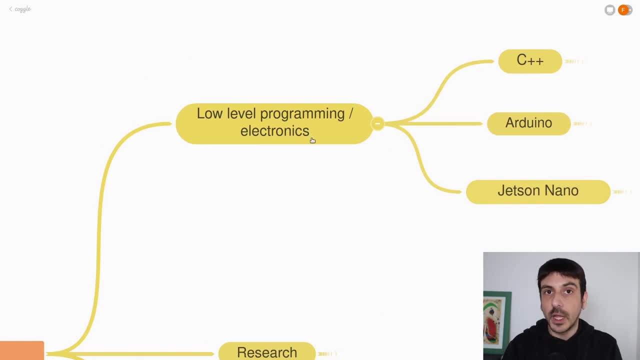 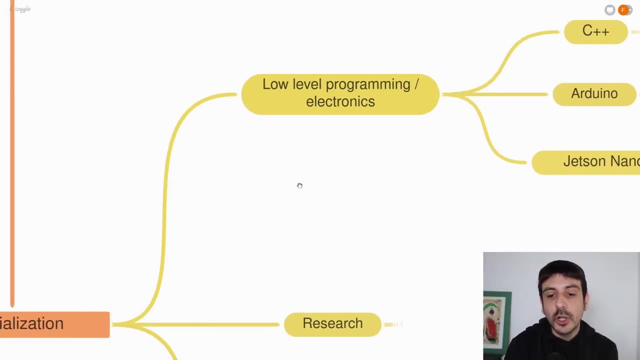 related to low-level programming or anything related to electronics. right, It's perfectly possible. So this is one of the ways in which you can specialize If you want to go deep into low-level programming, if you want to go deep into working with electronics, working with robotics. 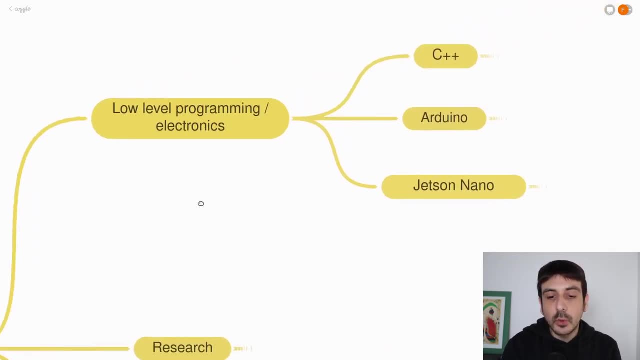 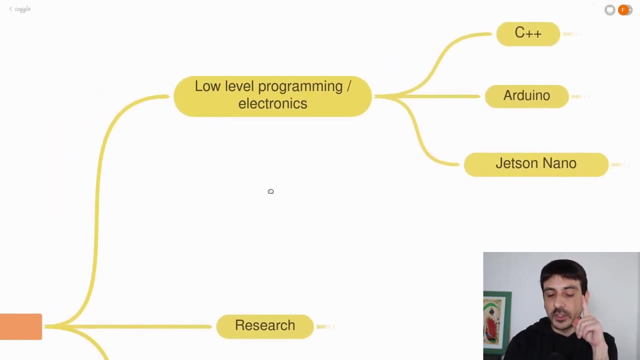 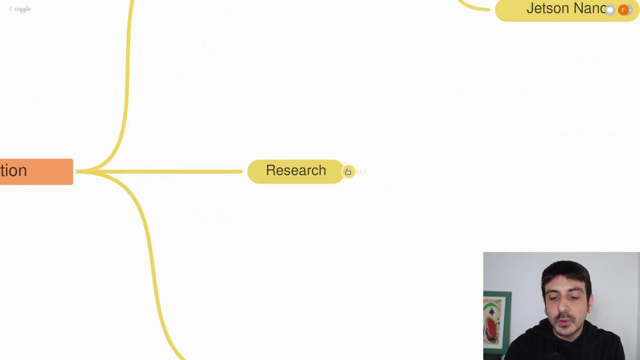 for example, then you can just specialize, and you can do it, Learning C++ and learning how to work with this type of edge devices. Now, another way in which you can specialize is by taking the research path right, By doing research, And this involves. 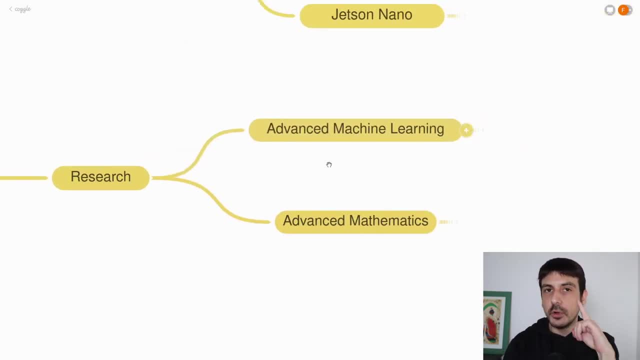 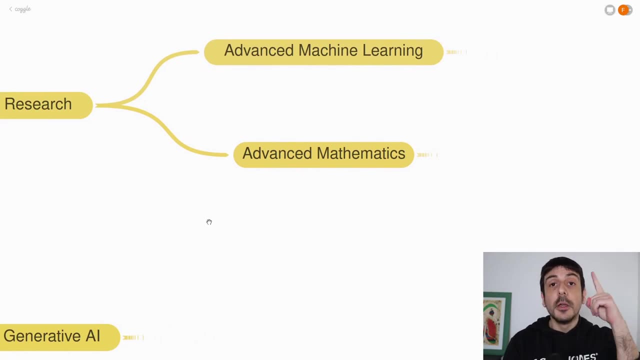 learning, very advanced machine learning and also very advanced mathematics. There's a huge misconception in computer vision, which is that you definitely need very advanced mathematics and you definitely need to know how to work with very advanced mathematics. So if you want to master some mathematical objects and operations in order to do computer vision- and that is not- 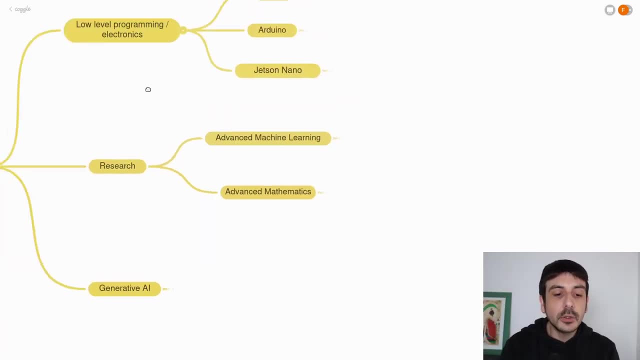 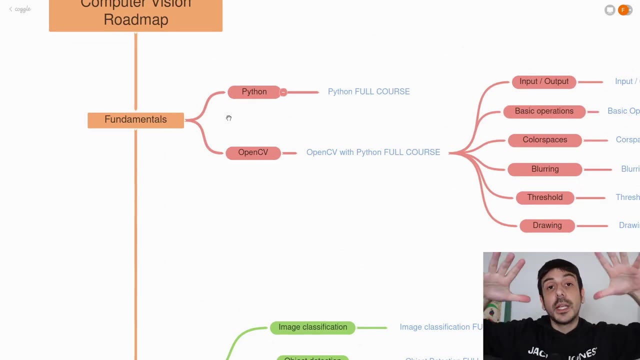 true. that's a misconception. that is false. I can tell you that you can definitely work in the field as a computer vision engineer and you can definitely take many, many projects. and you can definitely make a lot of money as a computer vision engineer by knowing Python, OpenCV and the 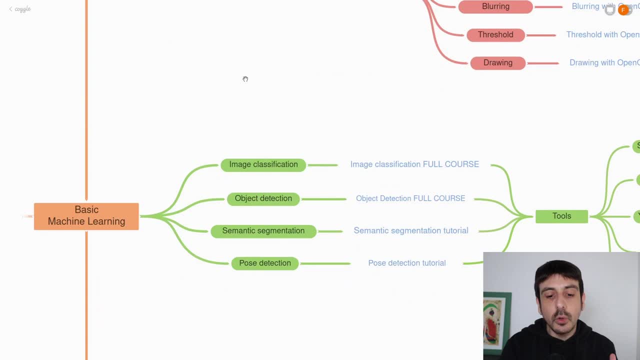 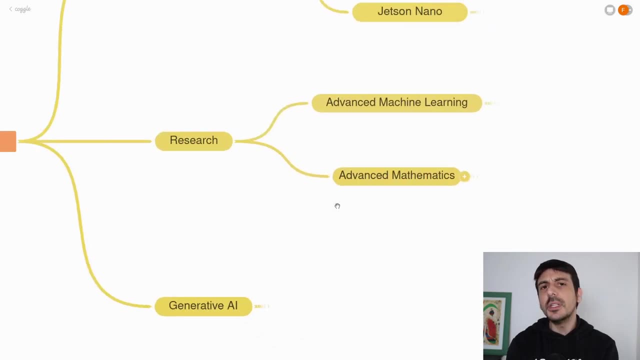 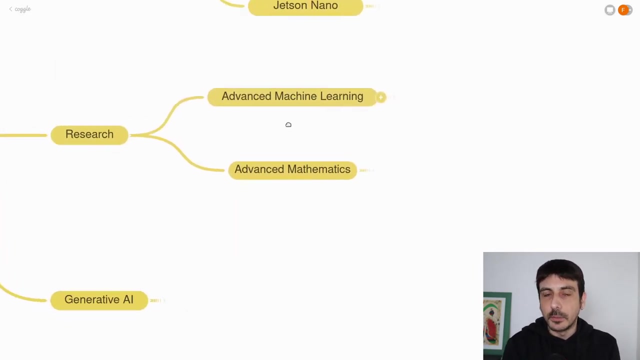 basics of machine learning. only by knowing this skills you will be able to solve the machine learning part of many, many, and you will be able to solve many projects knowing the advanced mathematics and the advanced machine learning and the advanced everything is not absolutely needed. that's why this is, i consider, 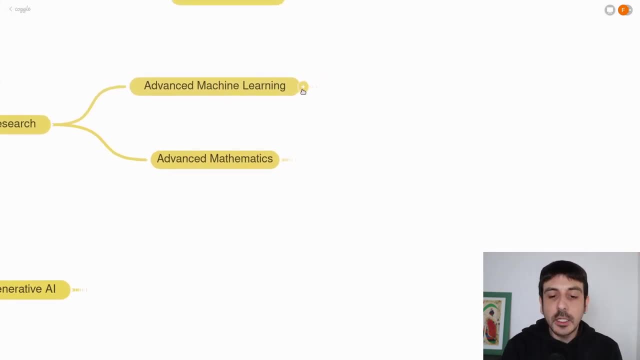 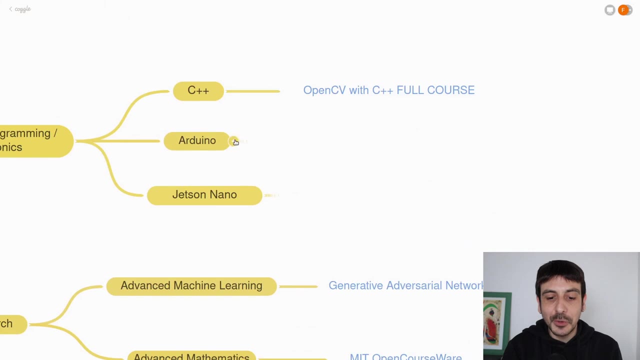 this is one of the ways in which you can specialize right and, if you want to take this route, these are some very specific resources you could take right and i forgot to mention these are some very specific resources you can follow in order to learn this other way to specialize in computer vision, which 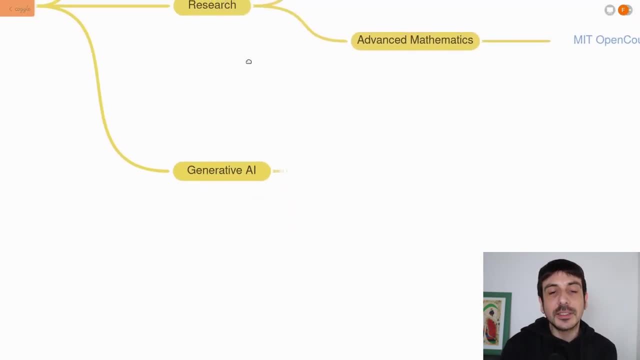 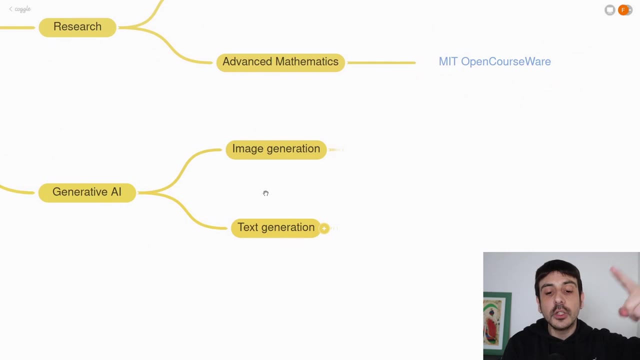 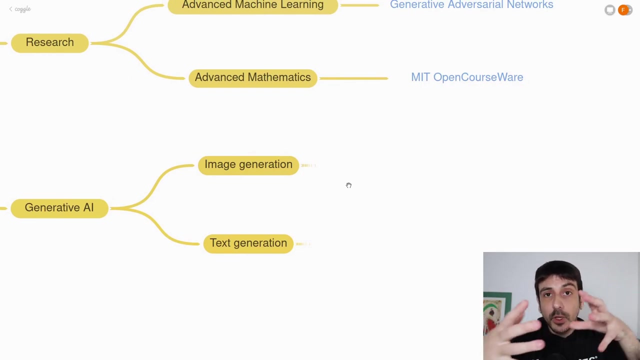 is low-level programming and electronics. but let's continue. now let's take it to the other way in which you can specialize, which is generative ai, and this basically involves image generation and also text generation. right, this is something that i would say it's huge already. it's already a. 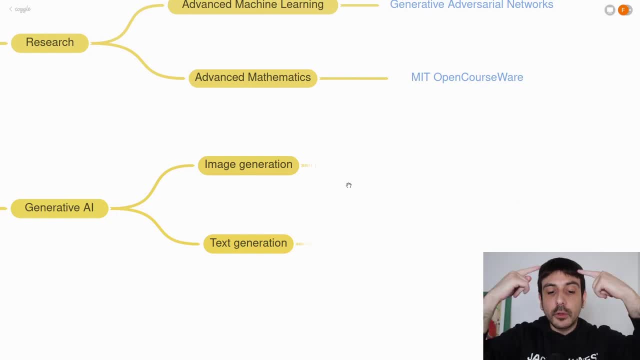 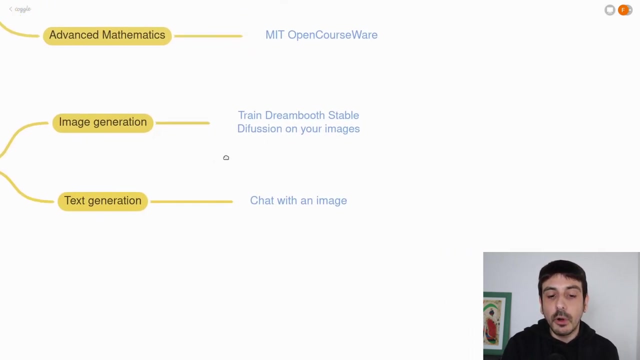 very, very important field in computer vision, and my thoughts are that in the next few years this is going to be bigger and bigger. this is going to be a very, very, very important field in computer vision, and this are some very specific tutorials from my own youtube channel you can take in order to learn. 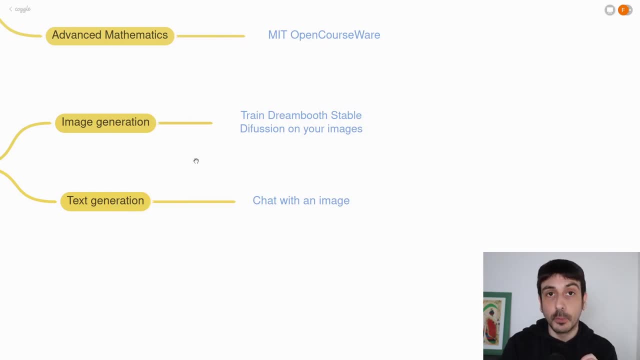 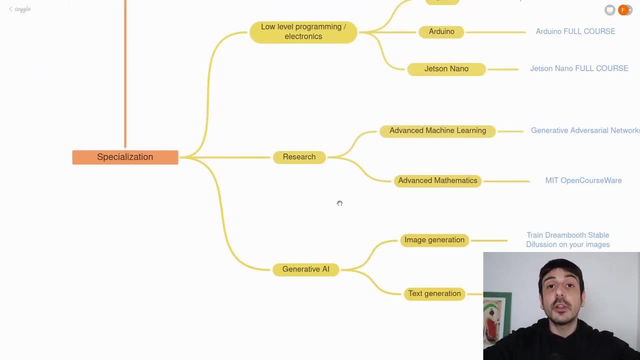 how to work with image generation and text generation in a computer vision project. now let's continue. these are some of the ways in which you can specialize in computer vision. these are definitely not all the ways in which you can specialize. there could be other ways, but i think 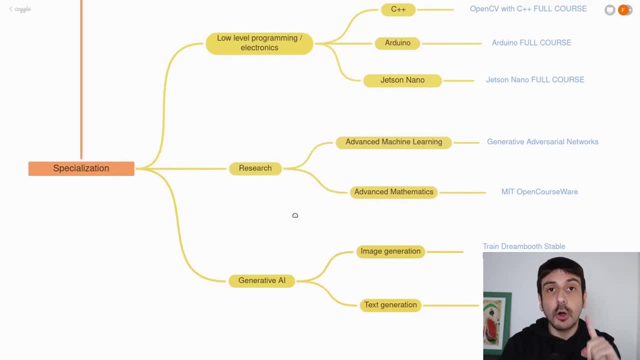 these are some of the most important paths you could take as a computer vision engineer. but now let's take it back. remember that from the beginning of computer vision, you can specialize in computer vision and text generation. right, and this is where we have all the basic machine learning we could take. 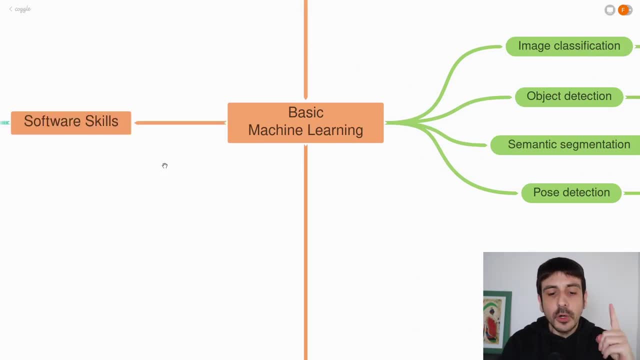 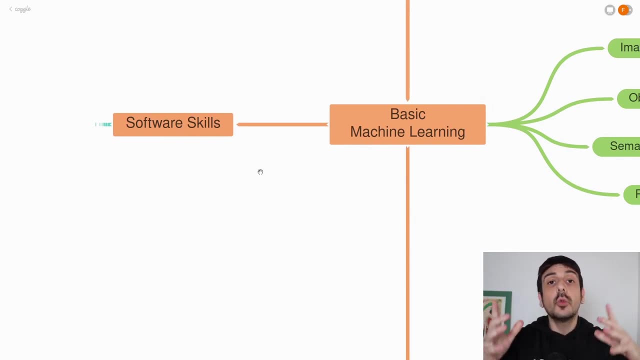 another path. right, let's see what's over here. and this is where we have all the software related skills. right, because, remember, as a computer vision engineer, you are not working on a vacuum. right, you are working with other software developers, you are building products, you are doing some things which. 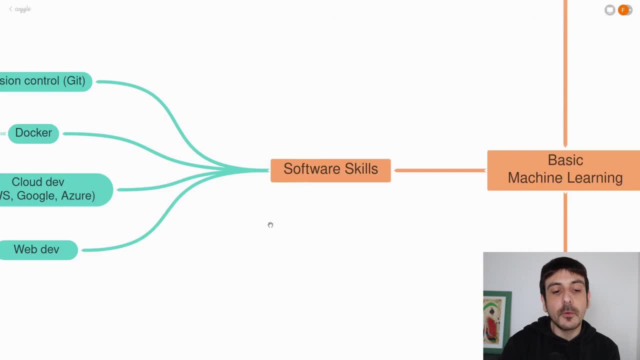 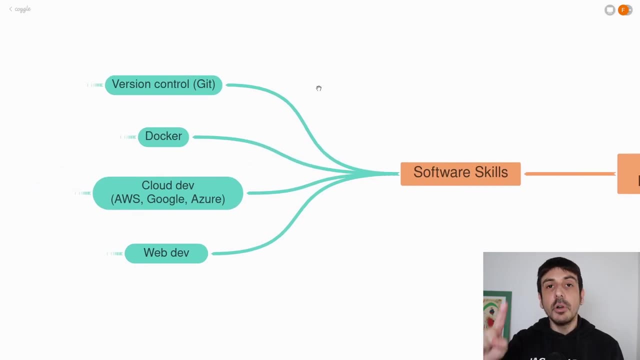 involve software. so the more you know about software, the more software related skills you may have is going to be much, much more better than what you are doing now. so i would say that i would say that i'm sure you will be well placed in that category if you're a computer vision engineer. 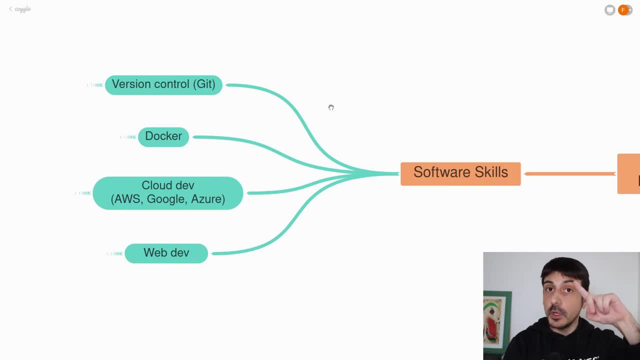 you do not have to do the work that i just mentioned, and why would you try and do some of the material we're going to be working on? i'm sure you will. it's important to know how you want to work in computer vision, and if it's not, it's only natural you work side by side. 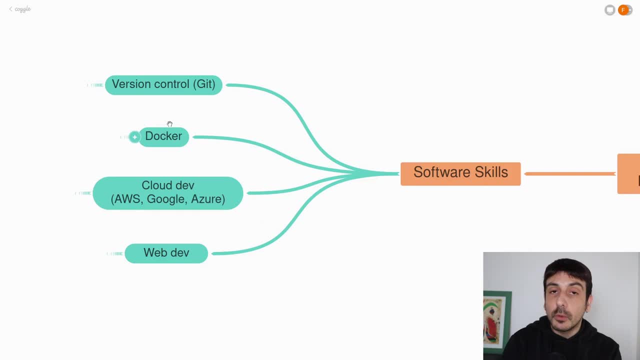 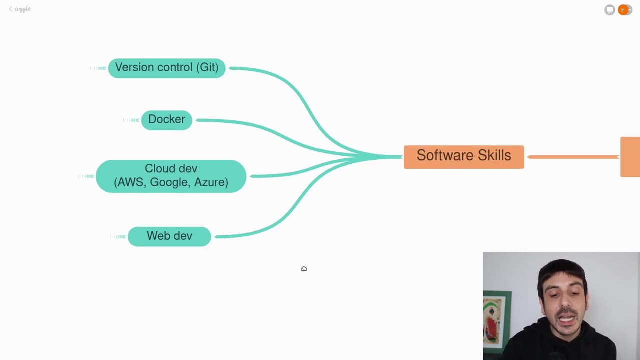 but in the future for you, if you get to code, basically the data you'll keep gathering and then other thingsこれは ένα file, because this is the native apple eness model case and i appreciate the aviation one, the winter version that you used to do. 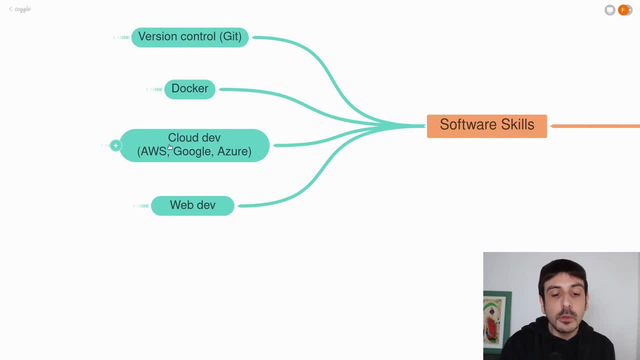 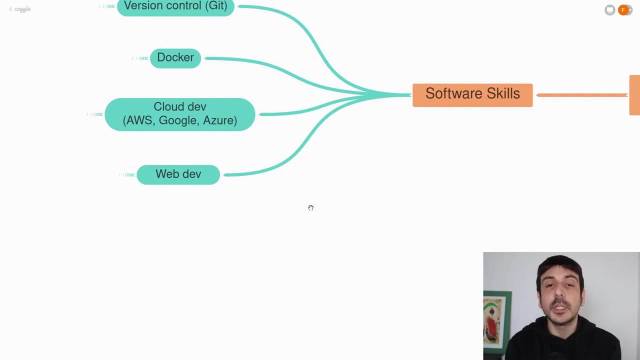 still still, uh, the overview. It's also a plus, it's something very important. if you are familiar with web development technologies, Let me tell you a very quick story about me, about myself. When I was just starting in computer vision, I completely underestimated how important it is. 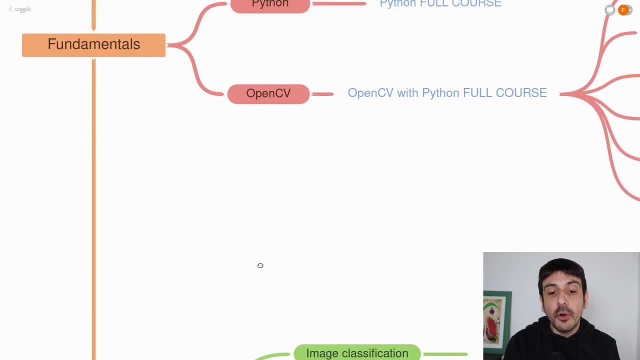 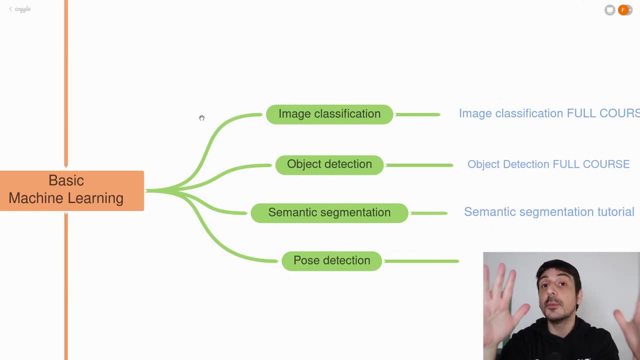 all these software-related skills and I thought that by learning Python, OpenCV and the very basics of machine learning- the very basics, by learning how to build an image classifier, the very basics of machine learning- I was all set. I was ready to work in the top companies in the field. 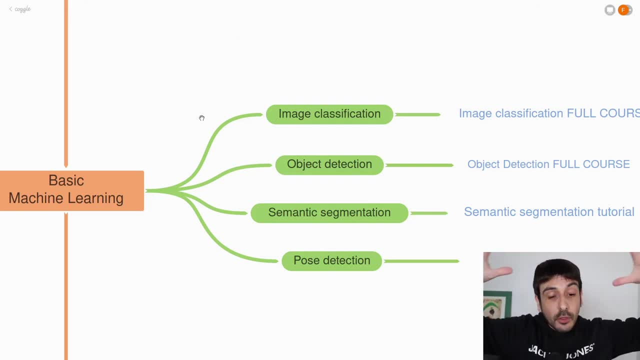 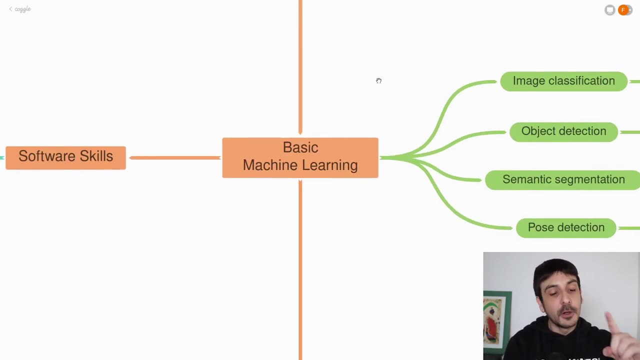 to work in Google, in Tesla, in SpaceX. I thought I was ready, that was all, that was it, and I was wrong. I was so, so, super wrong for many different reasons, and one of them is because I completely underestimated. 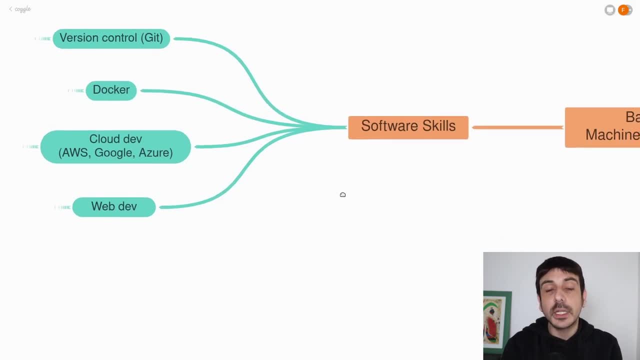 all these software-related skills. If you are going to work in computer vision, you definitely need to know something other than computer vision, And this is very important because this is very often underestimated by many people in the computer vision industry or in the machine learning industry. 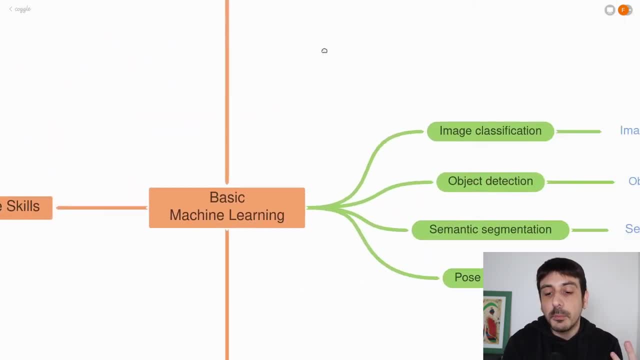 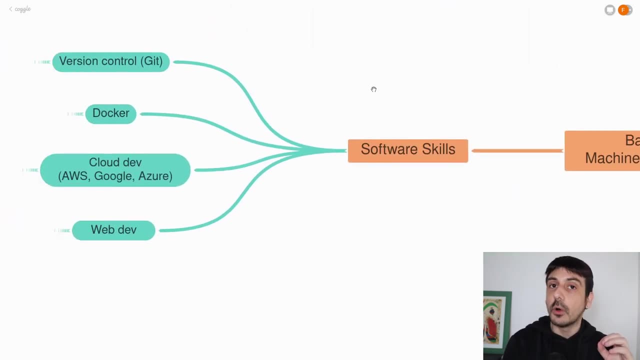 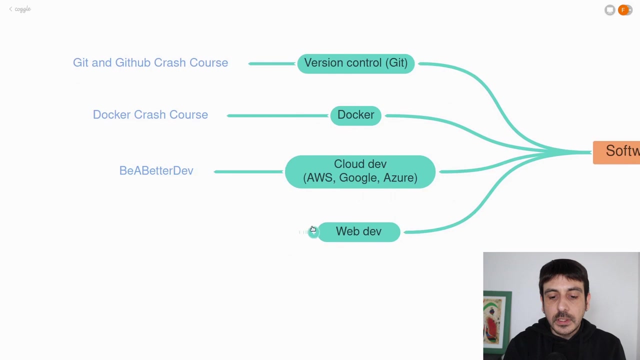 There are many people who believe, who think that by learning the basics of machine learning, that's it. That's not all. if you are going to work in the field, oh, you need to know something other than computer vision. And these are some very specific resources you could take in order to learn all these skills. 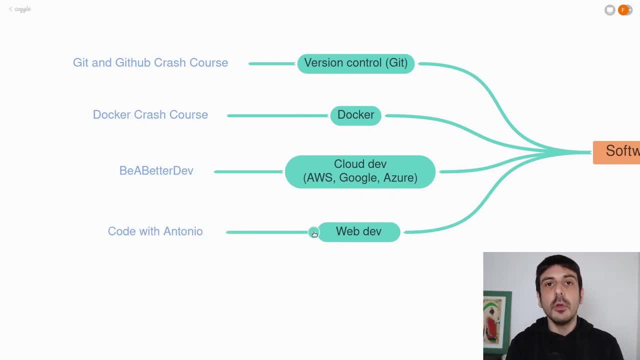 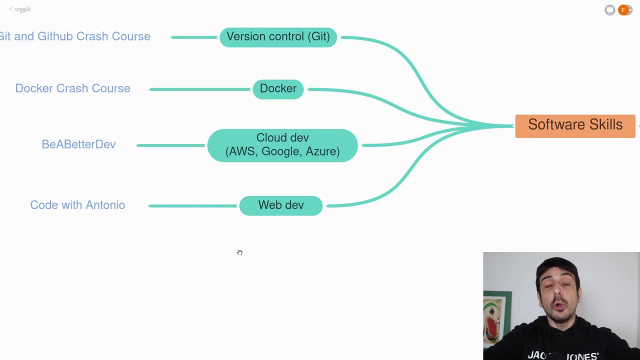 And also remember that working in a company as an employee, it's only one of the many, many different career choices you can take in your professional career. You could also be something like a freelancer, a freelance computer vision engineer, And if you decide to be a freelancer and a client hires you to do something like building a machine learning model, 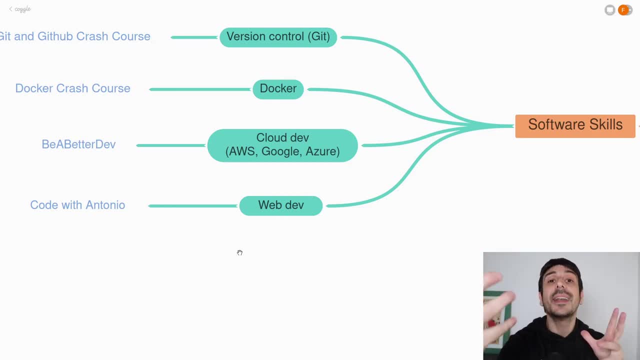 building an object detector and serving this model through an API, and you tell the client: okay, I can help you building the model, but in order to serve it through the API, I'm going to hire someone else, because I don't even know what's an API. 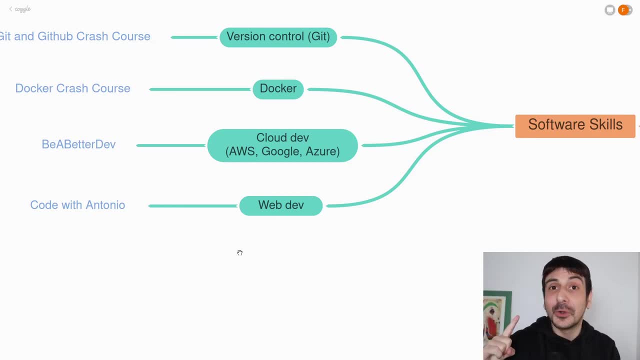 the client is going to say something like: oh, okay, okay, I am going to hire someone else. I'm going to hire someone else to do the entire project. It's going to be much more affordable. it's going to be much more easier to manage. 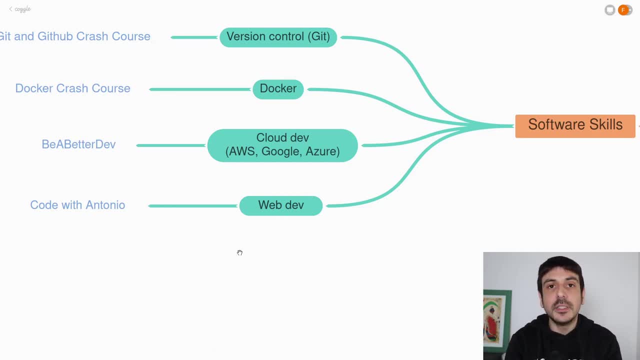 than if I hire many different developers to make each one of the tasks in this project. So this is especially the case if you decide to be something like a freelancer, because the moment you tell your client you don't know how to do something. 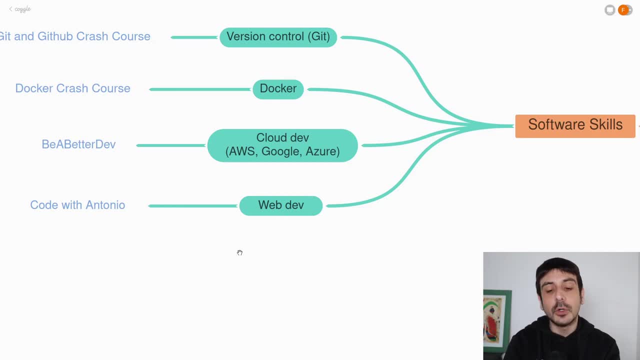 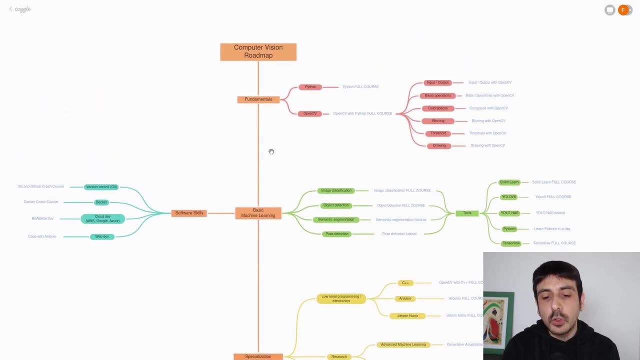 the moment, this client replaces you by someone else, So this is very important if you want to be a freelancer as well. Now let's continue. I have already shown you the entire roadmap you should take in order to become a computer vision engineer, with very specific resources. 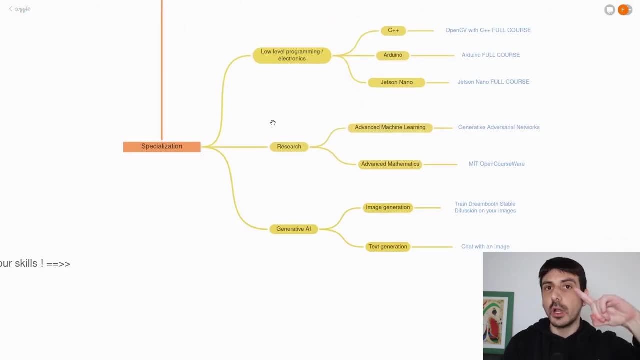 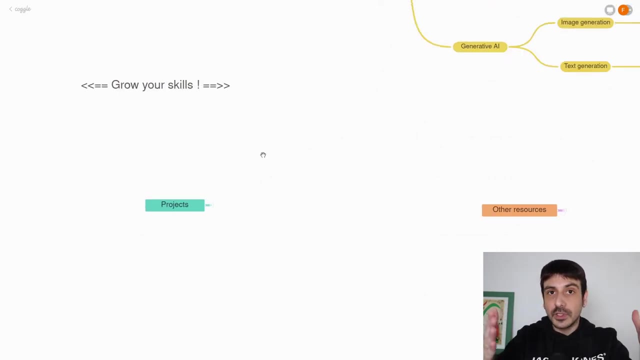 and I have also shown you all the different ways in which you can specialize as a computer vision engineer. Now let's continue, because now it's time to show you how to enhance your skillsets, how to grow your skills And one of the ways in which you can grow your skills as a computer vision engineer. 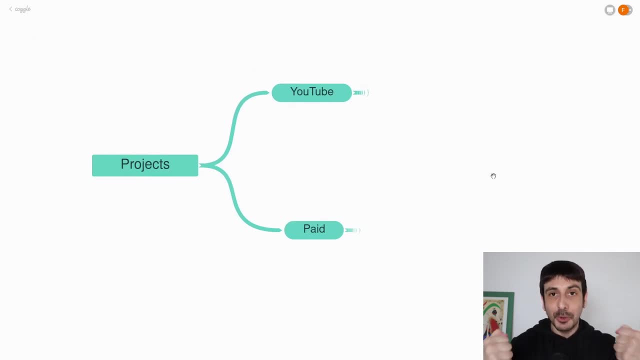 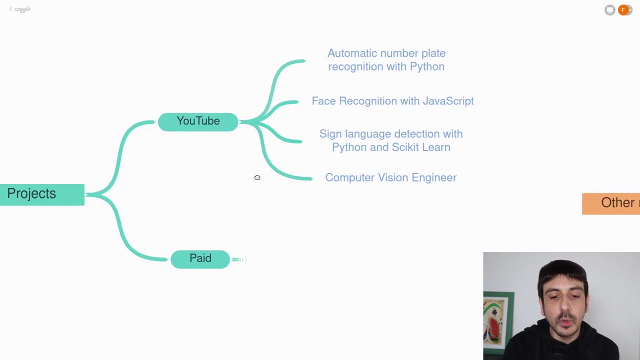 is by working on projects, by making projects, by doing projects, by having some experience working on projects, And there are two different ways in which you can do that. One of them is by following coding tutorials and projects in YouTube, and there are many, many, many projects you can take, you can do on YouTube. 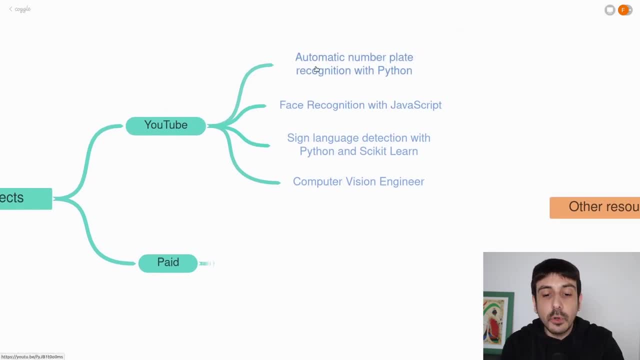 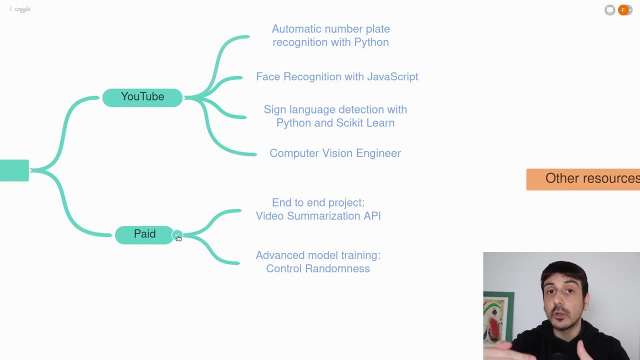 These are only a few examples of some of my tutorials, of my projects in this YouTube channel, And you can also take many, many projects. You can take many paid courses, right, If you want to take your skills a step further, if you really want to become like an absolute expert. 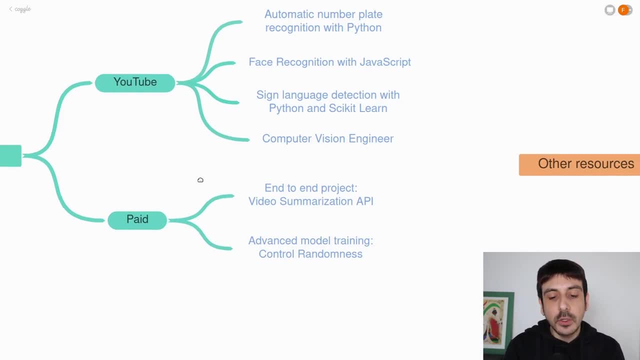 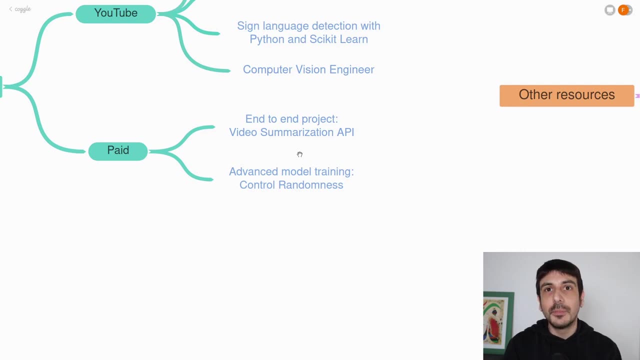 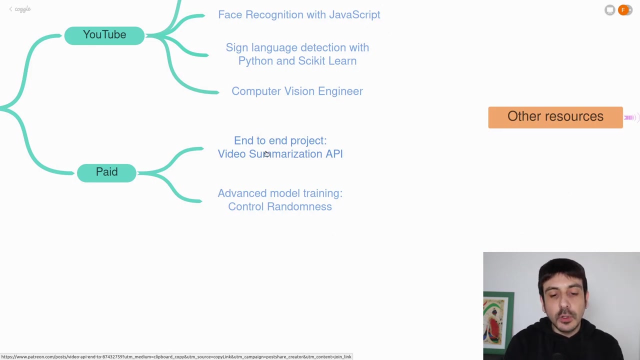 then you also have many paid resources you could use in order to enhance your skillsets even further. right, And these are only a few examples, also from my own paid products. For example, this is a project which is available in my Patreon, and in this project I show you the entire process of how to build a video summarization API. 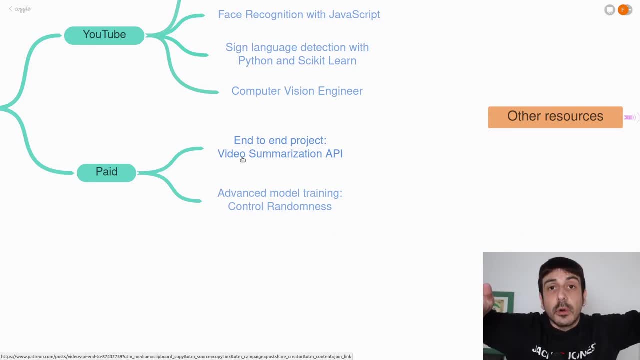 I thank you from the bottom of my heart And I show you the requirements up to the project deliverable and I show you every single step of this process: how to do the planning, how to do the system design, how to work in the execution. 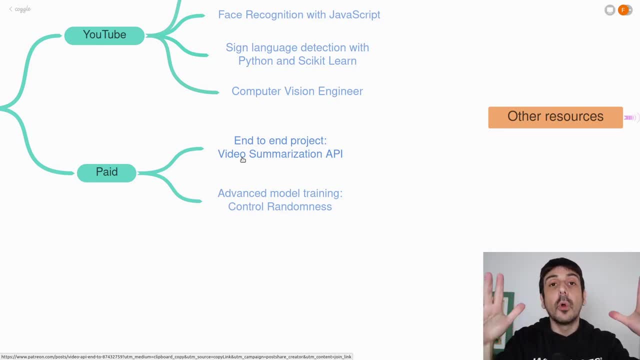 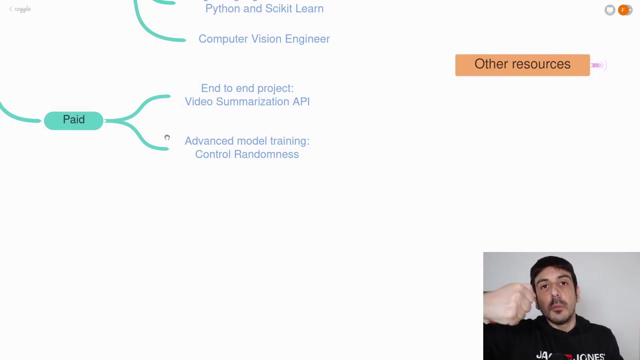 every single step of this process, and this is exactly how a real-world computer vision project looks like. Then this is another example that is also available in my Patreon, and this is a very advanced lesson on how to train a machine learning model, and it involves how to control the randomness when you are training a machine learning model. 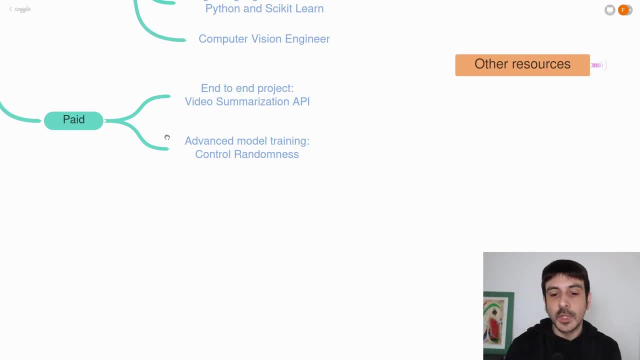 This is a very, very, very advanced lesson, And these are a few resources you could take in order to enhance your skillsets as a computer vision engineer. and then you also have other resources, and in these other resources are, for example, books. 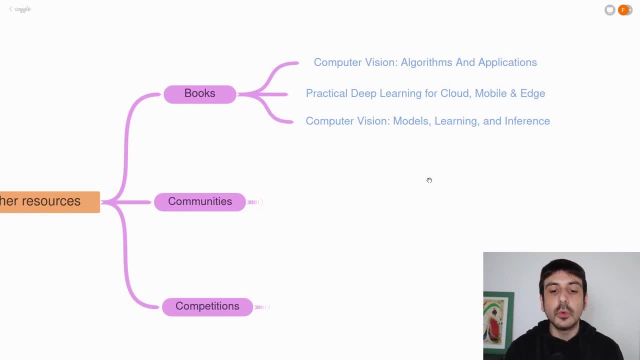 You could read books on computer vision in order to improve your skillsets as a computer vision engineer. These are only a few examples of some of the books you could read in order to become a super, an absolute expert computer vision engineer. Then another book: 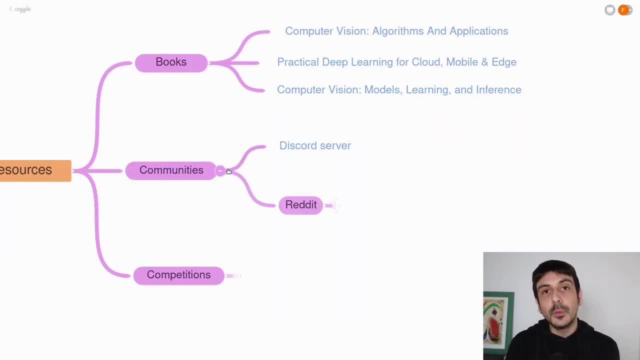 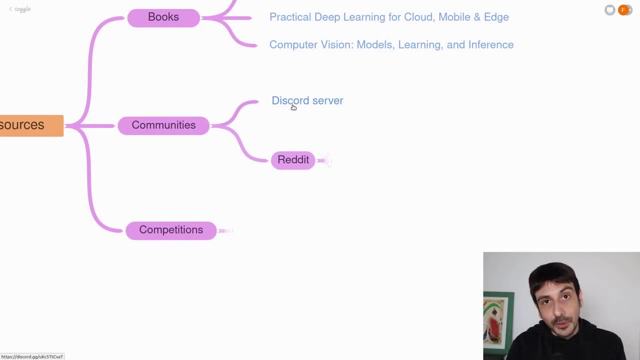 then another very interesting resource is joining a community, and these are some examples. This Discord server is this YouTube channel Discord server. right, This is our community and this is a very, very interesting resource. The way it usually works is that the members of our community post the projects in which they are currently working in. 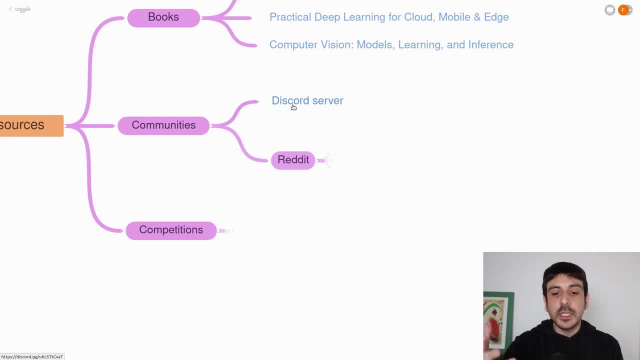 and everyone else recommends to this user different things he or she can do with his or her project. We say something like: Hey, have you tried to do this? Have you tried to do the other thing? Have you tried to do this with the data? 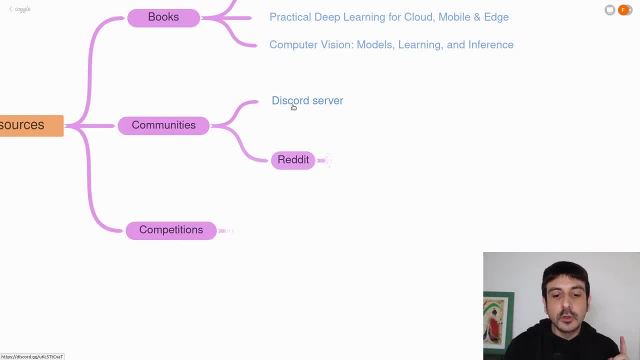 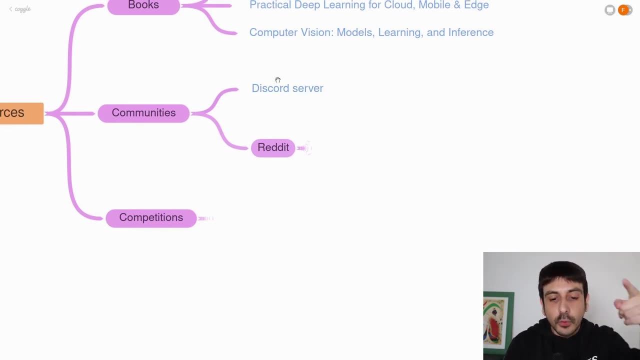 I don't know. We collaborate in many different ways, so we help everyone with their computer vision projects. This is a very, very, very interesting resource in order to go deeper into your knowledge of computer vision. Then these are some subreddits you will consider: computer vision, machine learning.